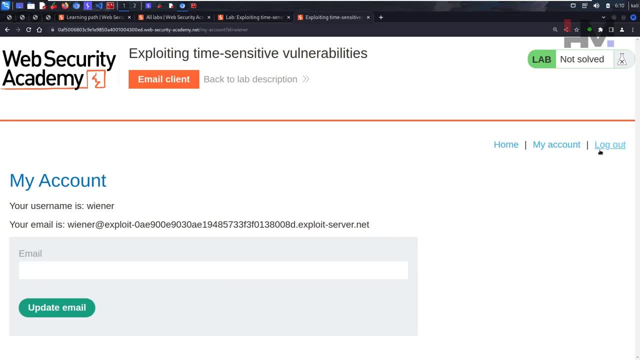 the application. Okay, So we have to log out. Okay, So we have to log out, We have to click the password. Okay, So by clicking this, you have to enter an email address or username. So we know the username, this one, right? So let's submit it and let's see what happens. So please check your. 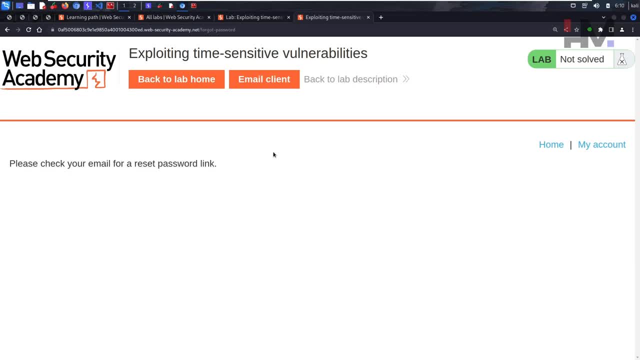 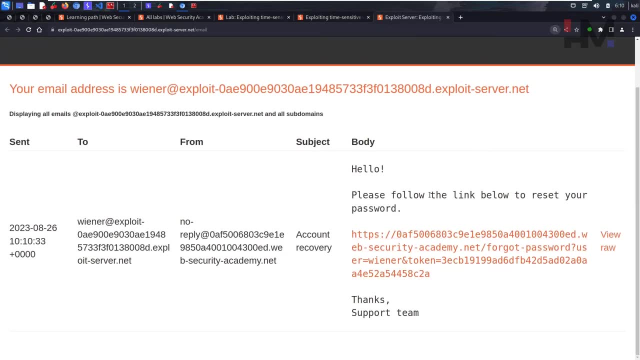 email for reset password link. So this will be our email client. Okay, So let's click this And, just as promised, we got a password reset link. Okay, So what does this password reset link actually contain? Okay, So, this endpoint which is forgot password and a user winner and token. 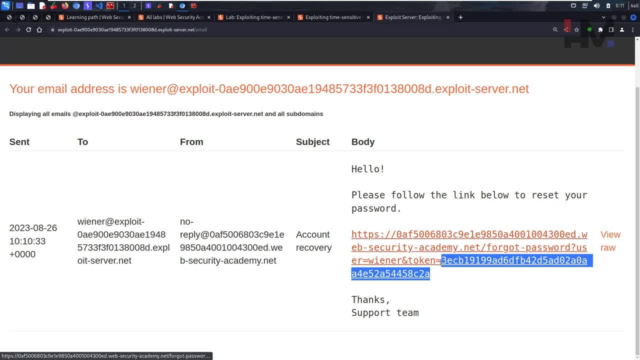 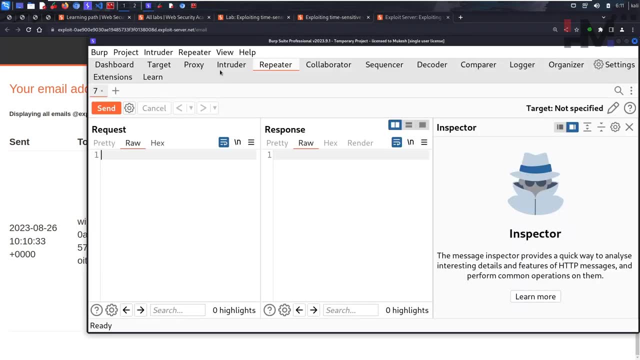 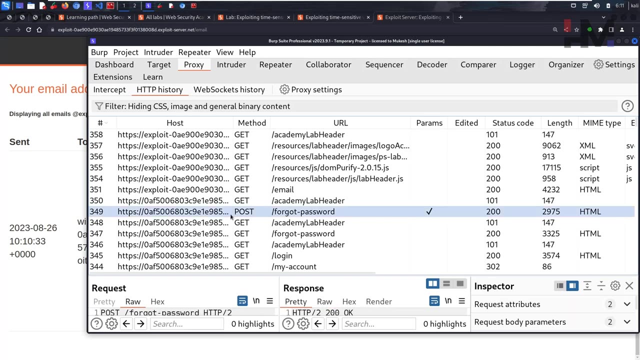 equals to something. Okay, So this is the token that we got. Hmm, Interesting. Let's go to Burp Street and let's see what we got. actually, Burp proxy. And, as you can see, this is the post request And this is the get request. Hmm, Interesting. 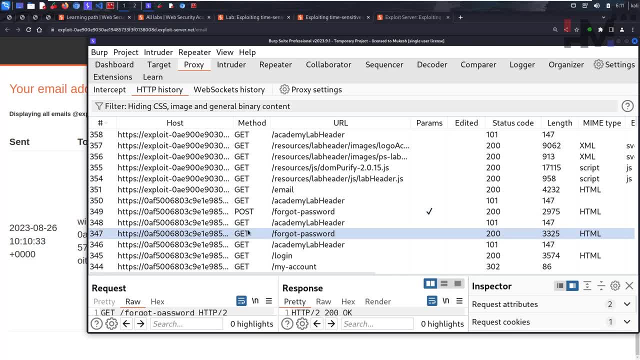 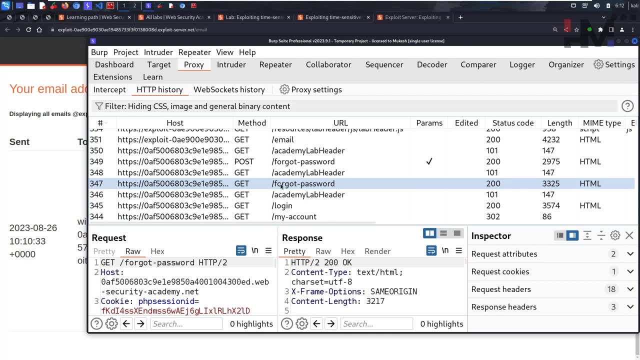 Okay. So do you understand the request methods like why post request and get request is: usually we do not send any kind of data. in get request- Okay, As you can see, the parameters are empty, but in post request we send some form of data. Okay, So in this particular case, we send. 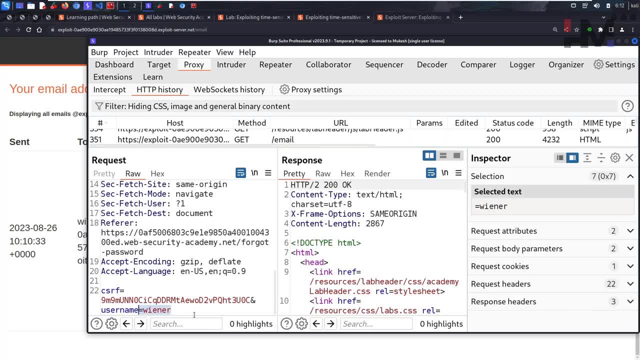 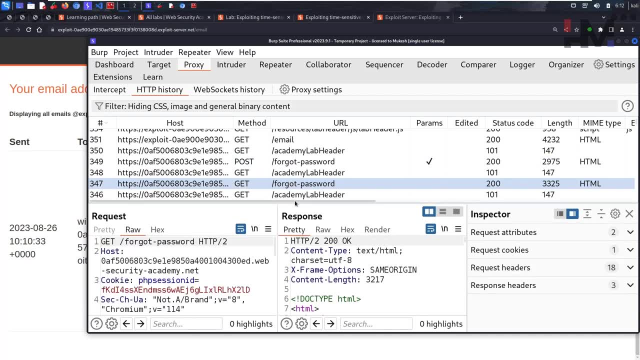 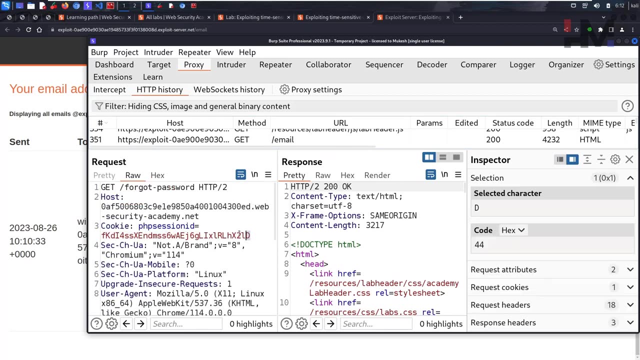 this particular username and CSRF token. We send these two things, Okay, So in get request, what do we get? Okay, I scroll down. I get nothing. Okay, So I'm not getting anything except this particular session ID. Okay, So what we can do is we can send both of them. 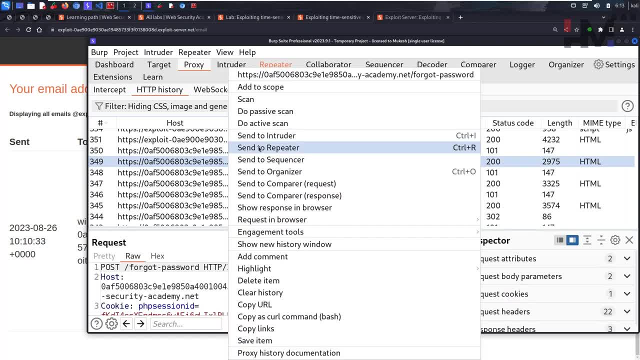 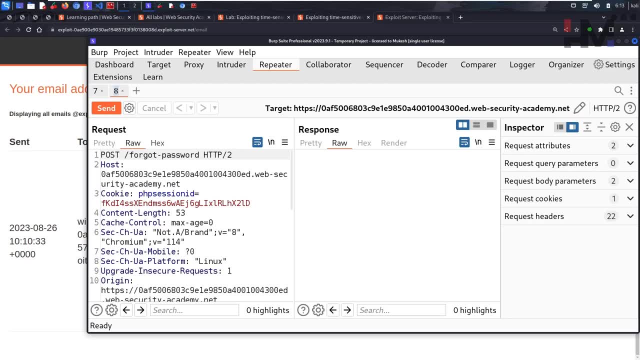 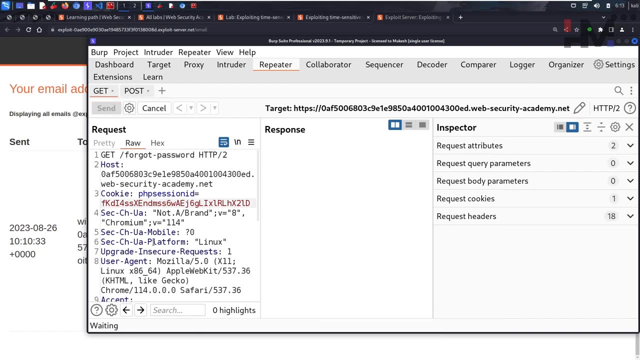 to repeater for testing. Okay, Although we need only one of them, So we will send both of them, Okay. So this is post request and this is get request request. Okay, If I send this request, what are the things that we are getting So in? 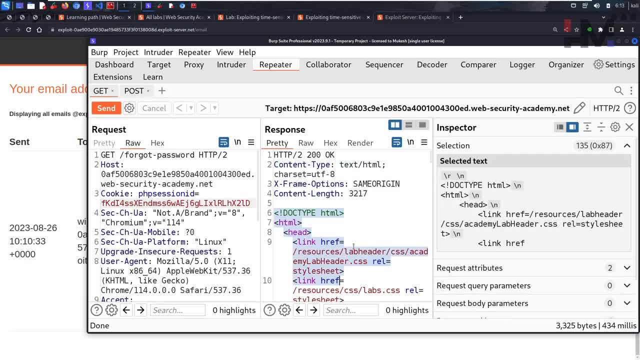 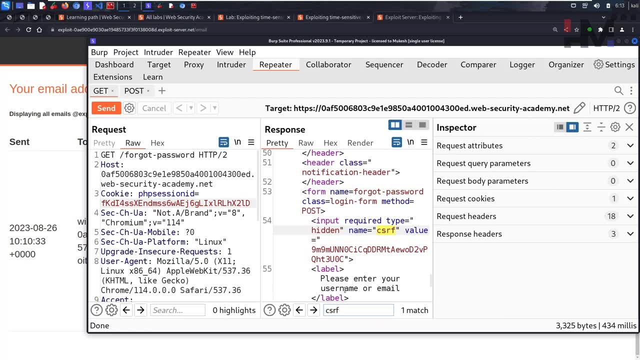 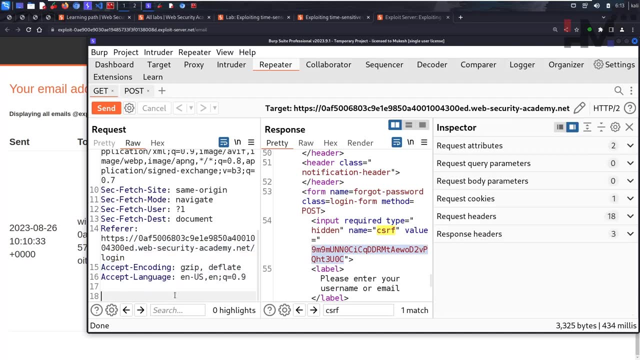 the header, we are not getting anything. And this is the document, which is a HTML page. We get something called a CSRF token. Okay, So this is the token we get when we are using get request. So we do not have any kind of CSRF token here. Okay, So when we send something, 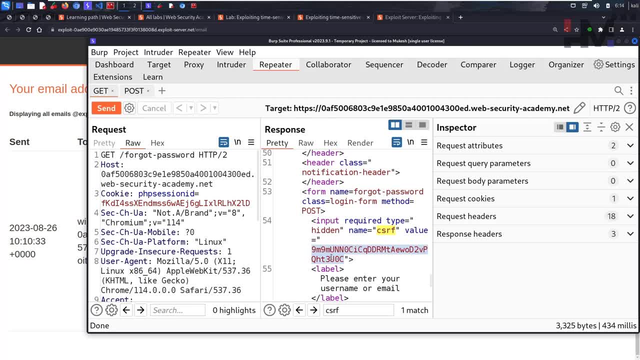 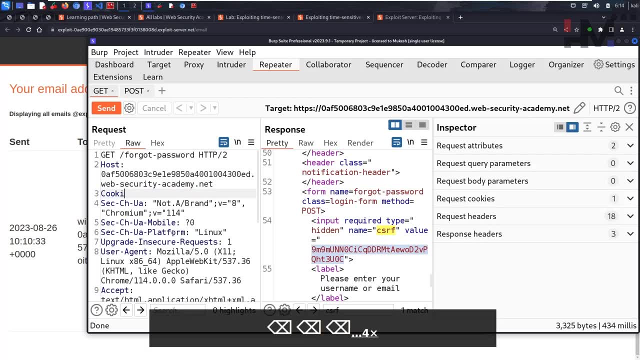 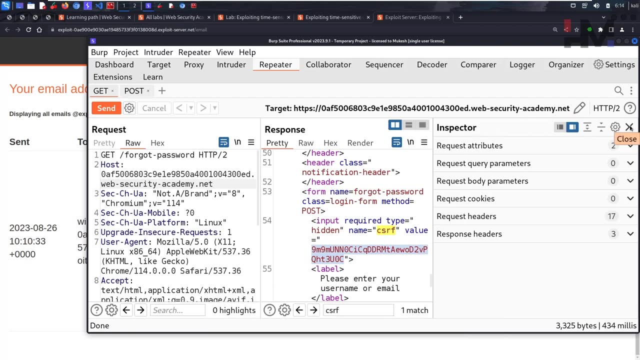 that we don't have, we get something that we don't have. Okay, So as simple as that. So if I try to remove this PHP session ID, so what's going to happen? Okay, So I should get a PHP session ID here, right? Let's see if it is right. Okay, So sending this, Okay. 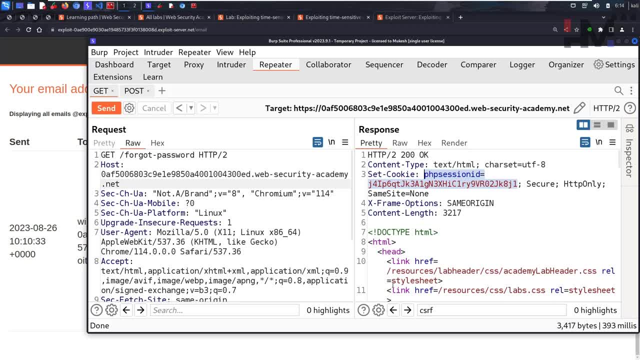 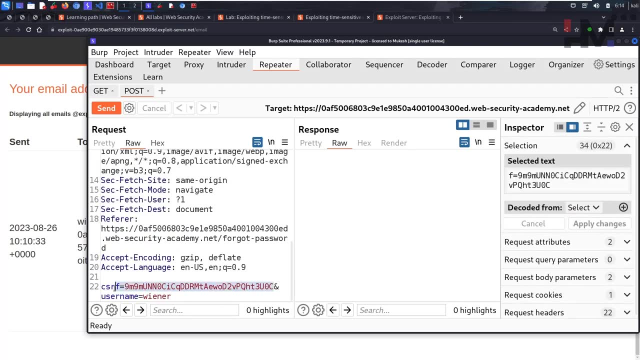 As you can see, we got PHP session ID here, Okay, So we can use this particular thing whenever we want, Okay, Right. So let's go to post request And, as you can see, we have a PHP session ID. We have a CSRF token- Okay, We have all all of these things. Okay, Right. 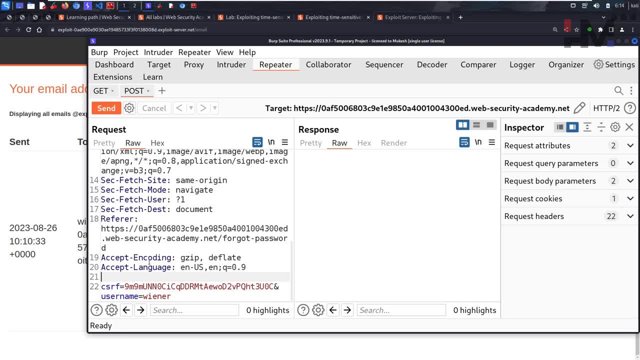 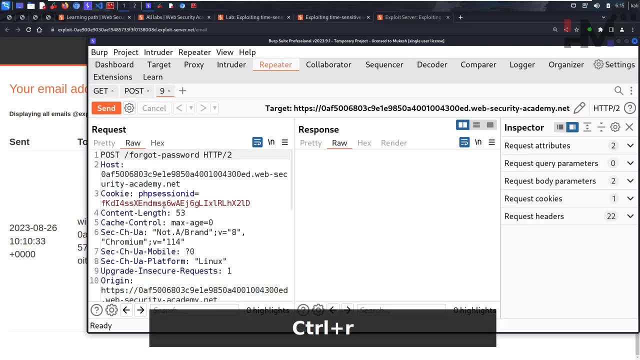 And what we can do is to test the race condition, we need at least more than one of the requests. Okay, So, let's make a duplicate out of this. Okay So, this is post Right. So what we can do is we can create a group with the both the post request. Okay, So what we can do, 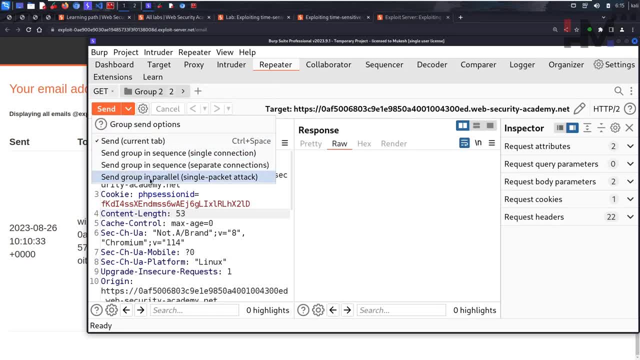 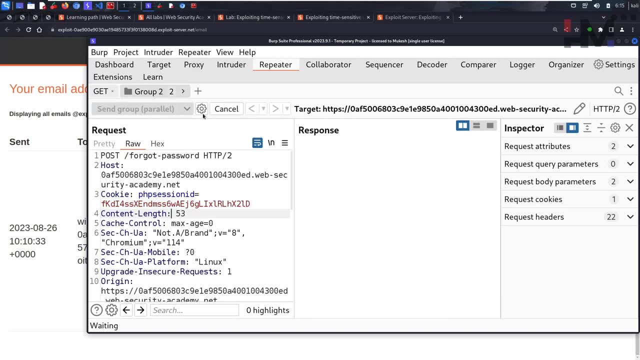 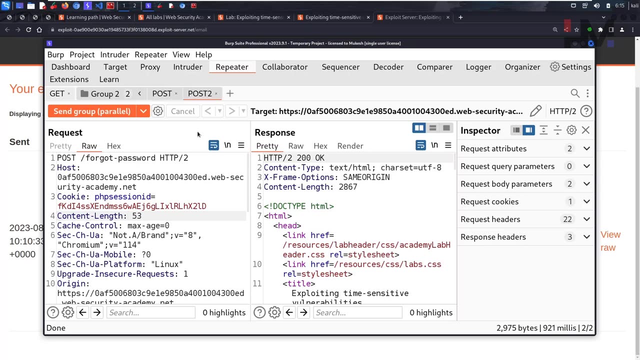 is, we can send this particular group as parallel. Okay, So let's see what happens. Okay, Sending the group. So it is taking me A lot of time, right? So let's see both the requests. So did we get anything different? 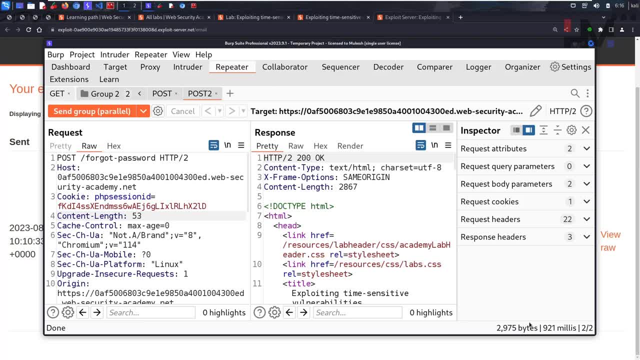 The only difference that we can see is this time right. So this is like 900 milliseconds and this is only like 600 milliseconds. What we can infer from this is this request came faster. Okay, This request came slower, which means they are going in sequential order. 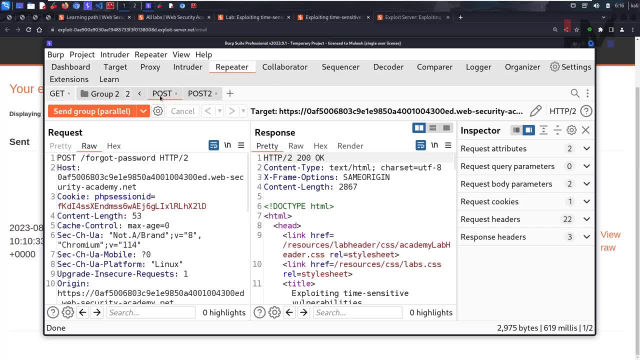 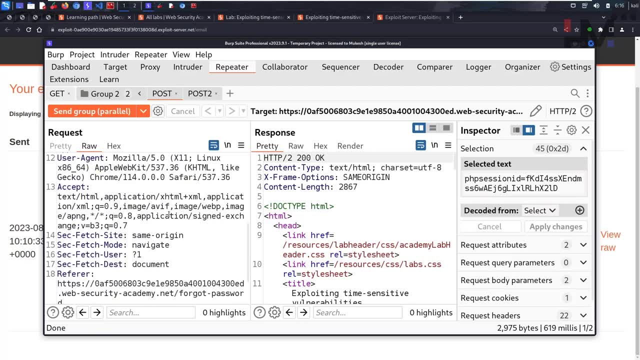 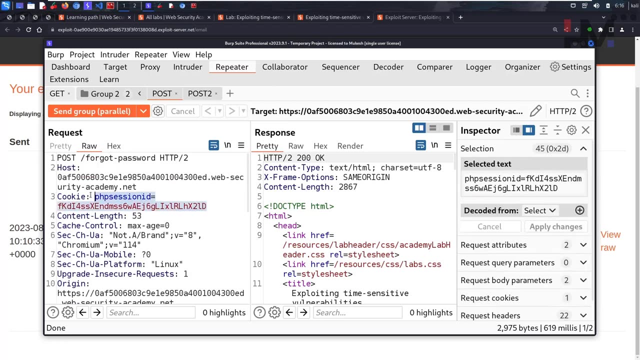 They are not going in parallel. So the main reason why they are going in sequence, what is? because of this particular session ID and CSRF token. Okay, So this is the main reason why, why they are doing a in sequential order, Okay, So what? 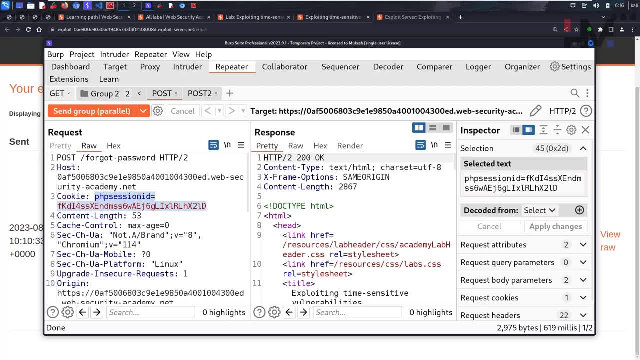 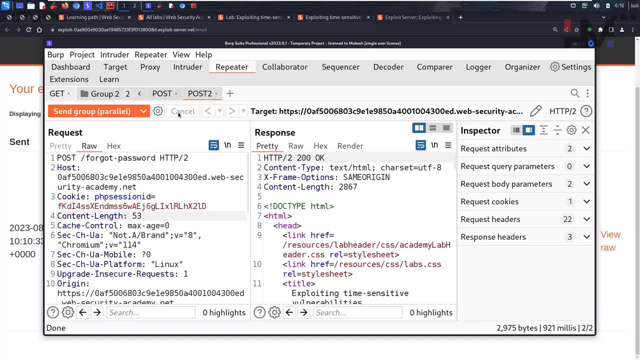 we can do is we can get a new CSRF token and a new PHP session ID and keep one of them. Okay, Not both of them, only one of them. Okay, We are telling server that both the request came from different sources. Okay, So this particular PHP session ID is different and which means this is a 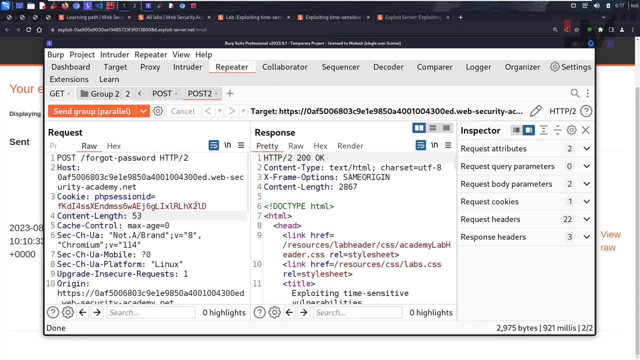 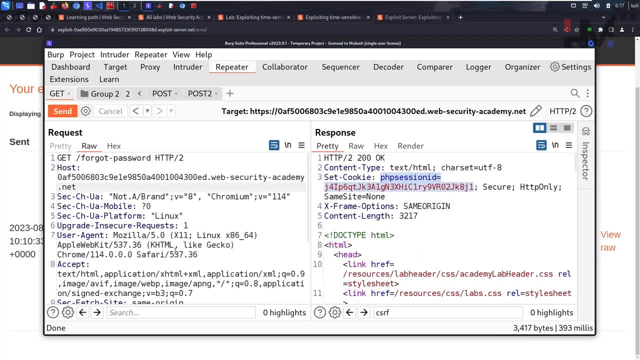 different user and this is a different user. So that is what we want to tell the server. Okay, So let's get a new PHP session ID and CSRF token. So it is easy, right? You delete the PHP session ID in get request And if you send it, you get a new PHP session ID. 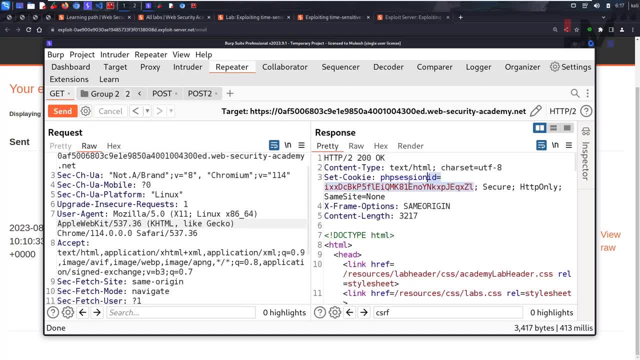 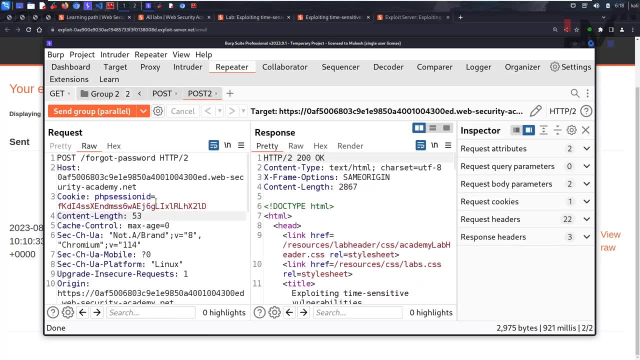 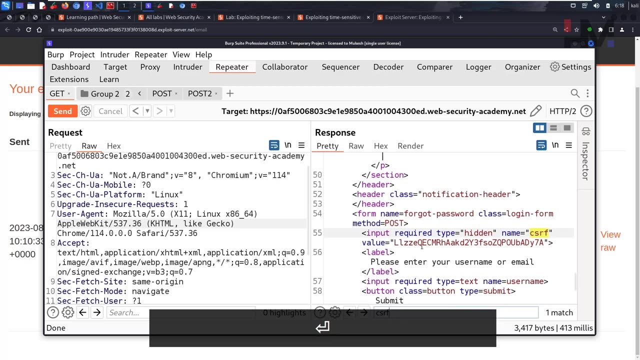 Okay, I'm going to get it again. Okay, We got something here, So just copy this one. Let's go to post two this time. Okay, Replace this and let's get the CSRF token as well. Okay, So this is the CSRF token. Control C. get to post two. 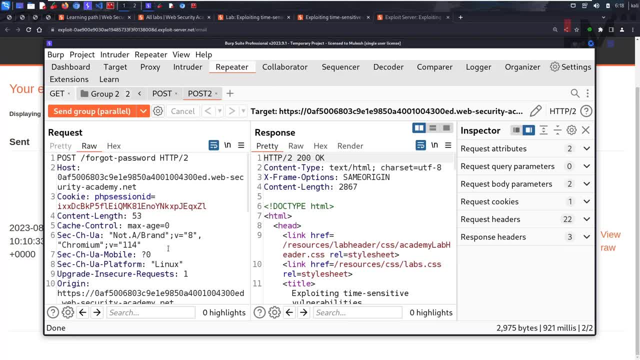 Okay, Control V. As per our theory, we should get both the request at the same time, right? So let's send them in parallel and see if our theory is correct. So this one is 600 milliseconds and let's see this one. So this one is also exactly the same time actually. 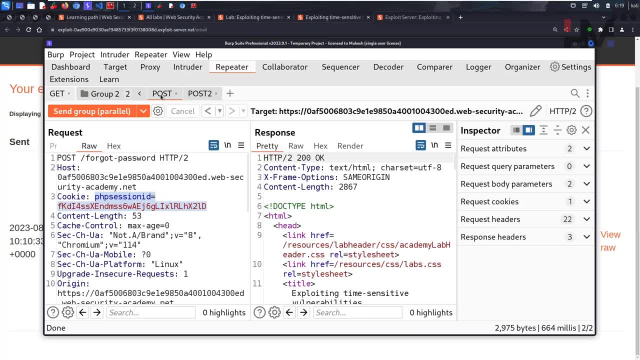 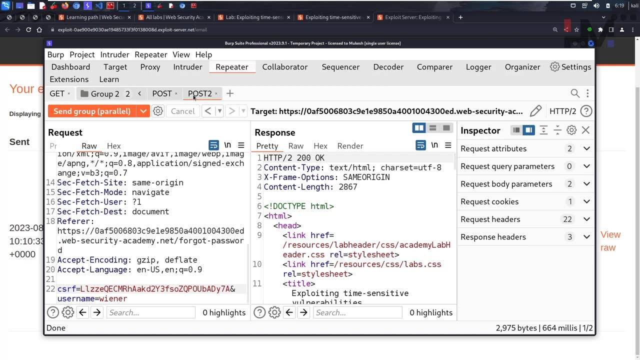 That is quite interesting. So, which means now the both the requests are going in parallel. So this is, This is exactly what we wanted. So the main part is: did we get the race condition? Okay? By race condition, What we mean is so both of them should have same token, Okay, Same. 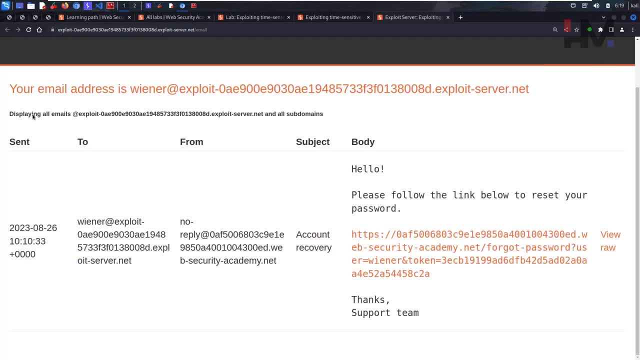 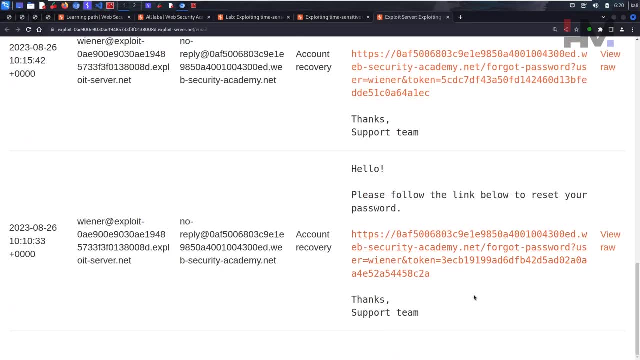 reset token, which will be displayed in the email address Right. So if I just reload this, I can see that previous emails, So this one is like our first email. Okay, Single post request. Okay, So next time, what we did is we sent. 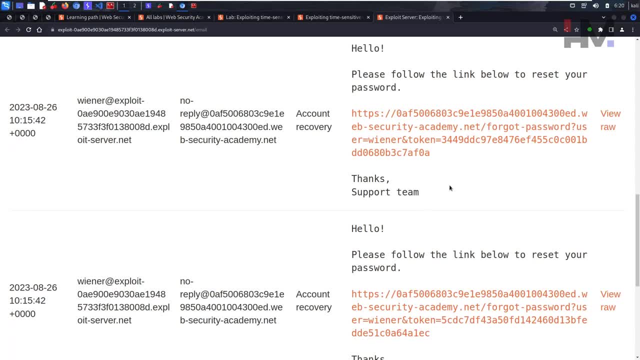 two requests at the same time, but one of them is like 600 milliseconds and second one is like 900 milliseconds. okay, so in that case, what happened is it received two different tokens. so next time we identified it and we rectified it and we sent both the requests at the same time. 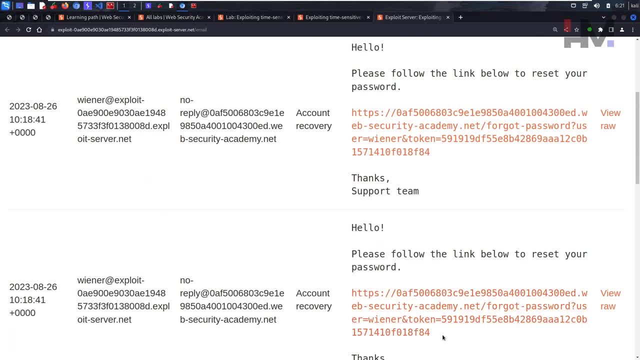 so let's see this time what happened. so this time, as you can see, both have the same token, okay, which is quite interesting. so this tells us that there is a race condition in this particular case, right, so what we can do is we can exploit this by sending two different users, okay. 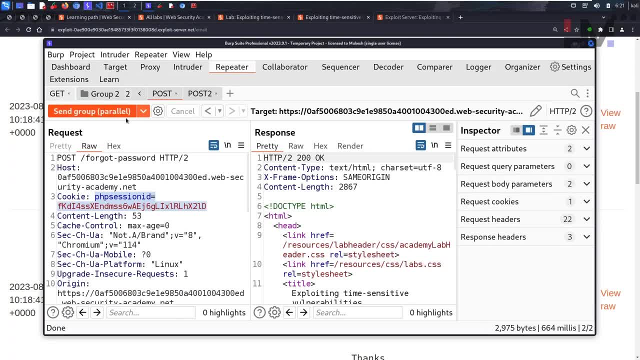 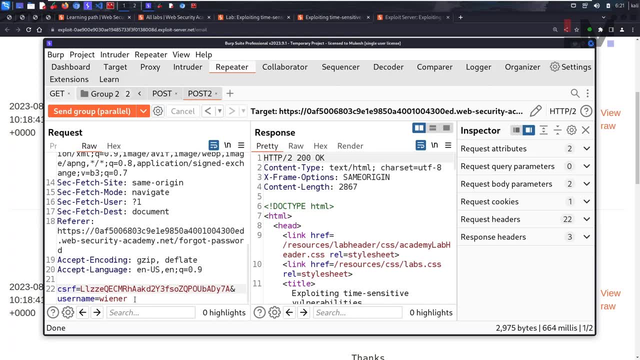 say something like: one is wiener user and one is carlos user. okay, so what's going to happen then? so what's going to happen is, during the generation of the token, both are at the same time, so we can exploit this by sending two different users. okay, so? 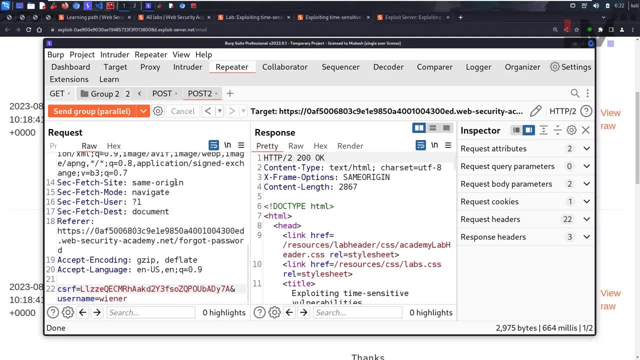 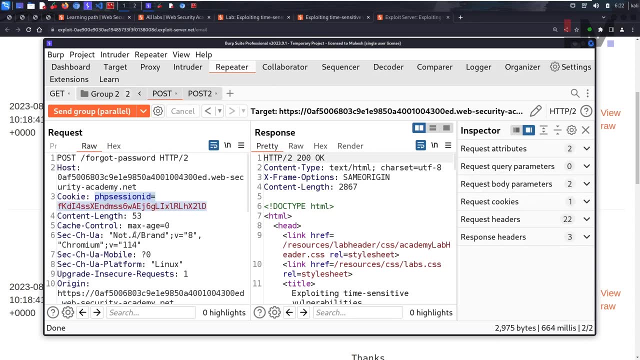 same place, okay, like a same race window. so what happens is both of them receive same token, so we will have a carlos's token and wiener's token as same. okay, so when we get same token, what we can do is we can simply use the token and we get the solution okay. 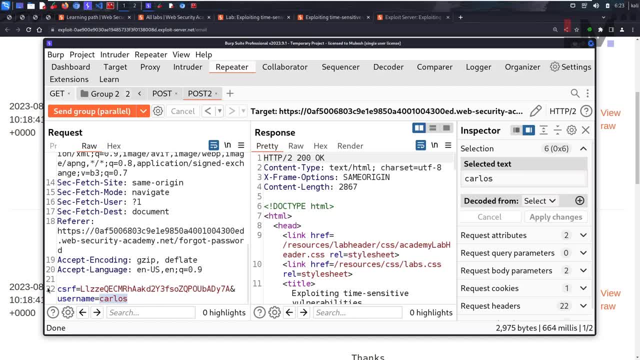 so it is as simple as that. so i just changed the user name to carlos, which means that this carlos is a random, and it is specified as a new token, which means that this carlos is a random user sending this particular request, and this one is sent by wiener user. okay, so what we are essentially. 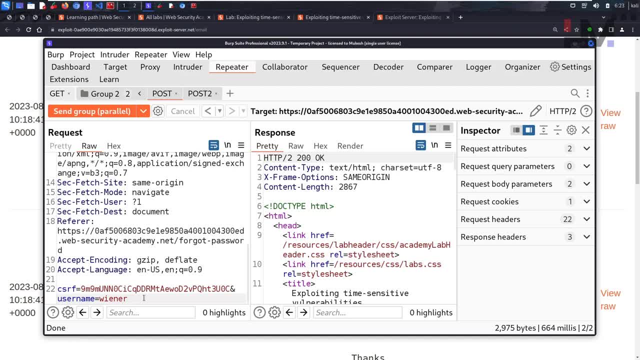 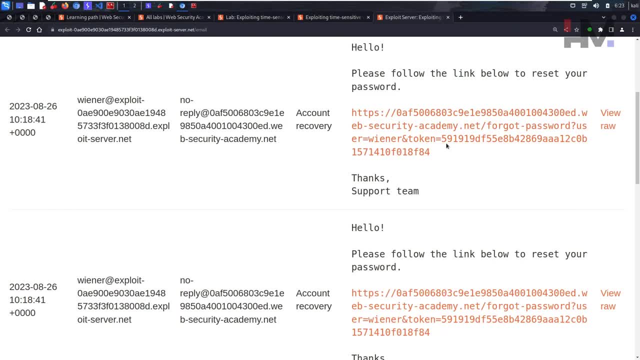 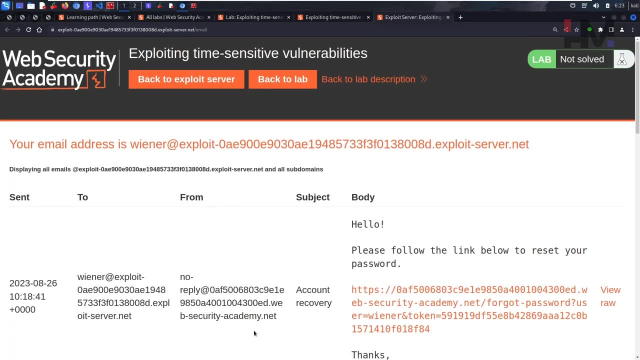 doing is we are creating two users that want to reach the server at the same time, and both will generate same token, just like we did before. okay, so we can only get one of the request back to us and we can use that particular token to change carlos's password. okay, so that's what we want to. 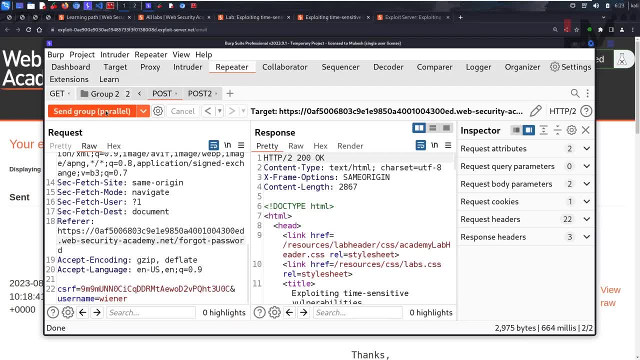 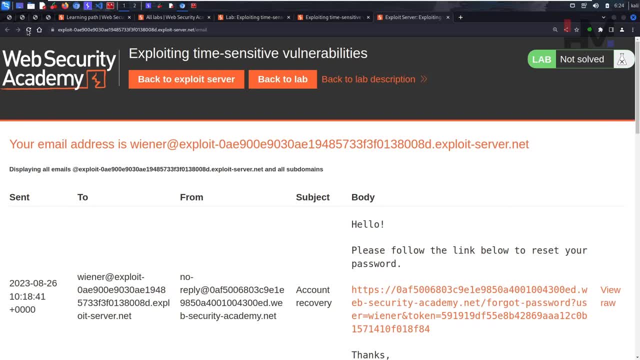 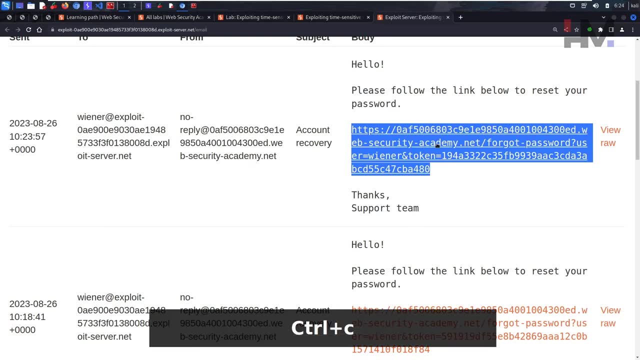 do right. so let's send this and let's see what happens in the email client. what's going to happen? we are only going to get one email, which is wiener's email, which has a user wiener. so this is quite expected, right? so what we will do is we will not click this one. okay, if we click this one.